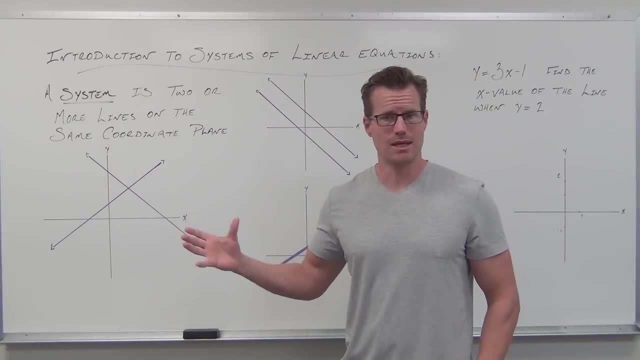 talking about two lines on the same graph. That's really it. Now, if you think about that, what are the three ways you could really have two lines, or more than two lines, on the same graph. Well, two lines, they could either cross or not cross, or be the same line. That's. 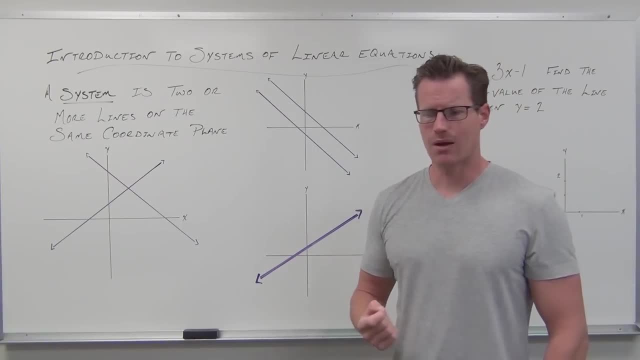 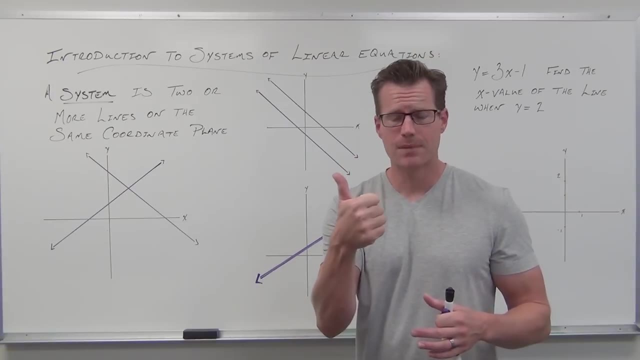 the three cases we have with systems of linear equations. Now, as we unpack the next several videos, what's going to happen is I'm going to show you how to solve systems graphically. that's method one, then with something called the substitution method, much, much more elegant. 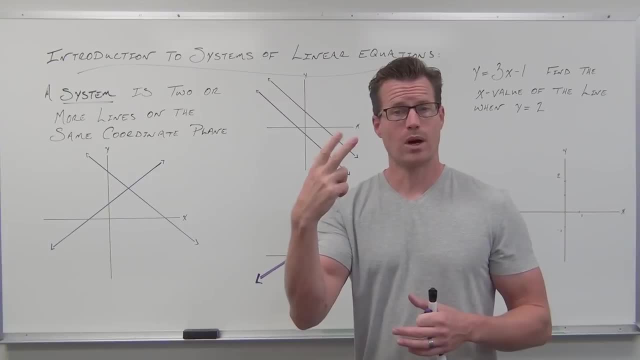 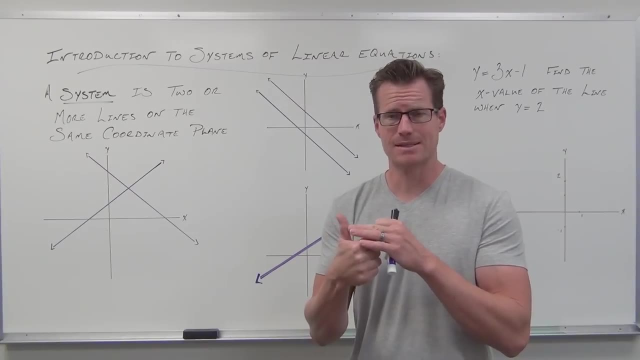 and then with something called the elimination method. The last two are where we're trying to get to The first one. we're going to learn really fast that it's not our best method. It takes a long time and it's not that accurate. You're always constantly having to check your work. 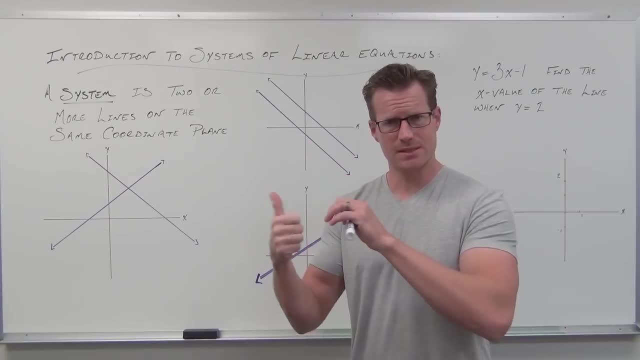 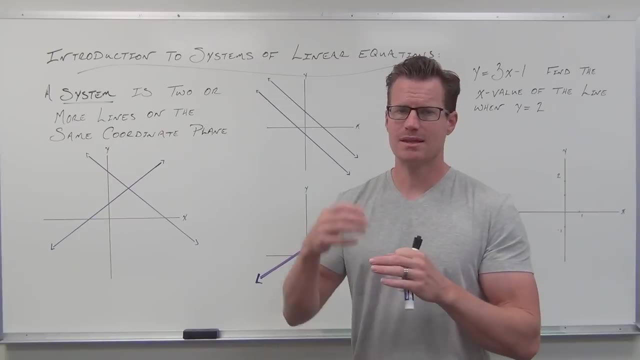 So this one, this is just to get us somewhere. okay, These couple videos here about the graphing method for solving systems of linear equations is just to get the idea in your head of what is actually going on, because it's really useless to talk about the substitution method. 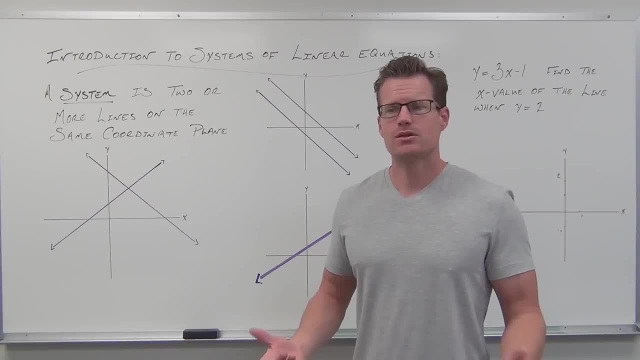 and elimination method if you don't really get what's going on. So here's what's going on. We have these two lines on a graph, or we have these two equations that are going to make two lines on a graph. Here's your one thing You're looking for where those 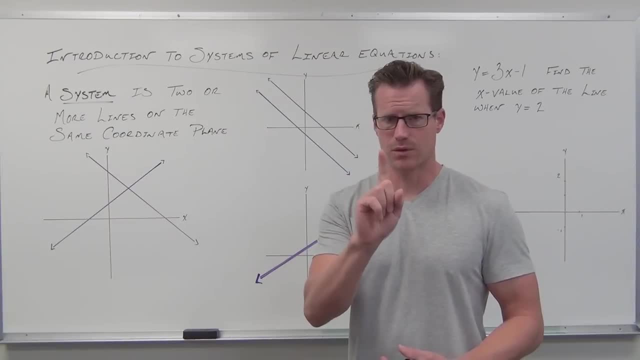 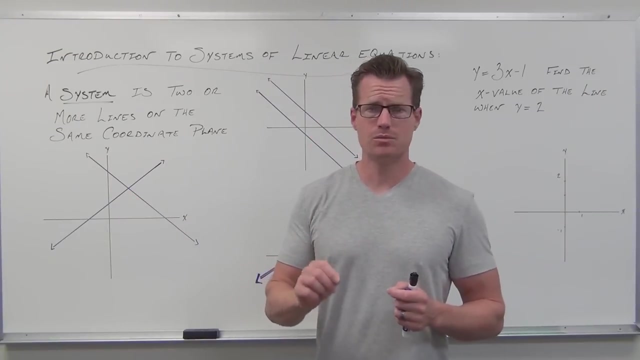 lines cross. You're looking for the one point where those lines cross. Well, could you point to it? I'm guessing you could if you were just looking at it. That's the point where these two lines cross. It's the one point in the world that is common to both lines. 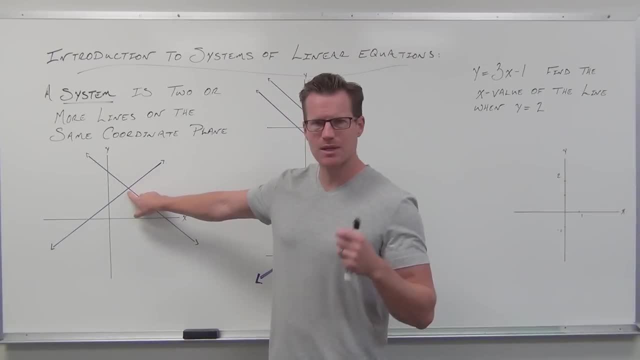 That's interesting, right? That's the one point that you could possibly have. that's on both of them. That's what an intersection means. is this point that's common to both lines or both curves, or both graphs, or both functions or both linear equations here? 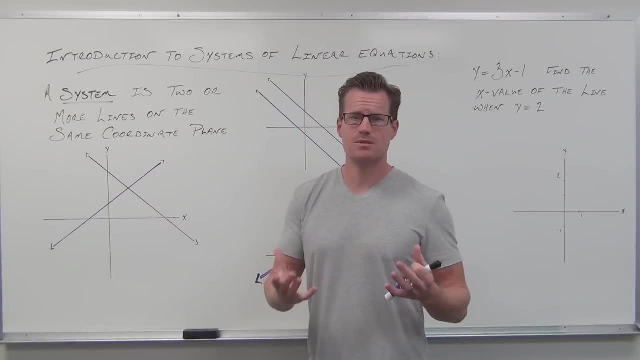 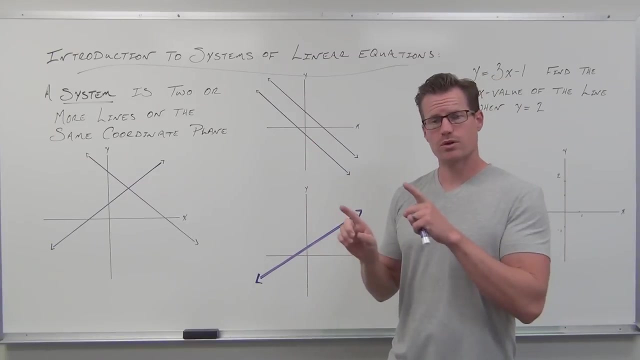 So our goal in this whole exploration of systems of linear equations is: find that point. Now, if that's our goal, are there times when we can't accomplish our goal? Yes, That's what these two situations say. Remember: if you have parallel lines, you're never going to cross. Those lines are never. 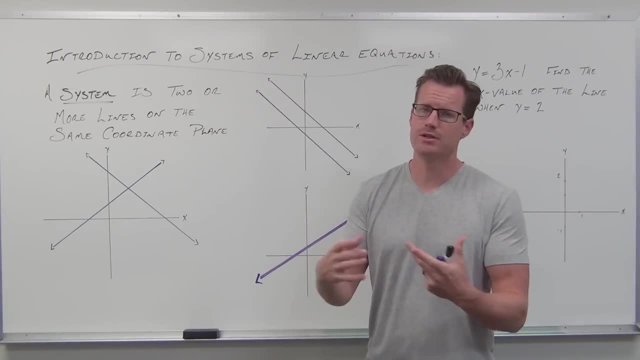 going to touch. Therefore there is no point. that's common to both lines. So if they're not crossing, they're not intersecting. there's no solution to a system of linear equations if you have parallel lines. It's interesting Remember what parallel lines meant. I hope. 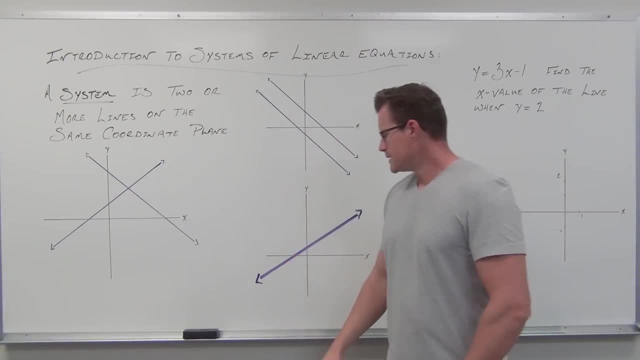 you do. Parallel lines mean this idea of same slope. Now the last case. What if you graphed a line and you graphed the exact same line on top of it? That'd be pretty redundant. you're going to intersect at every point. That has an infinite number of solutions. 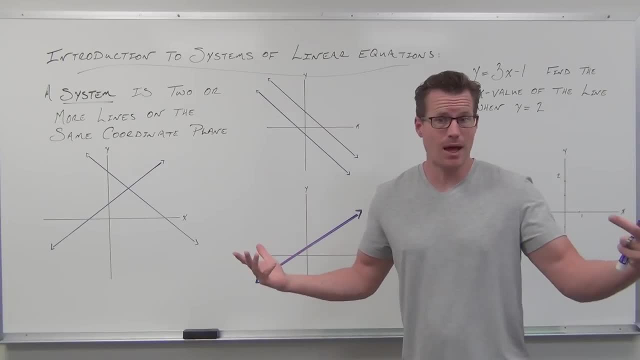 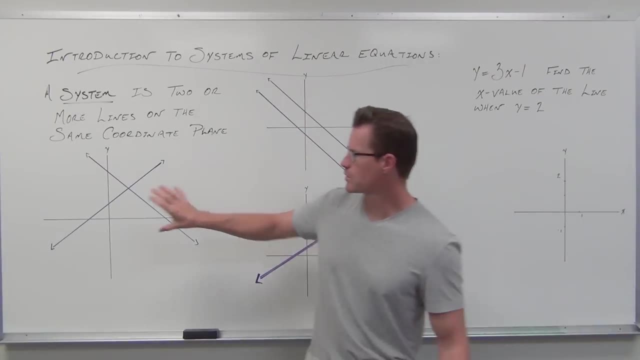 because at every single point you go: yeah, I'm on both lines. Obviously I mean the same line. so how could I, how could I not be? That's what that is. So here's our three cases for systems. The first one, this is the one we're looking for almost all the 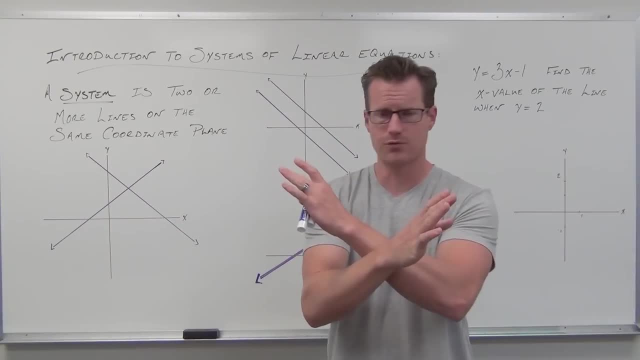 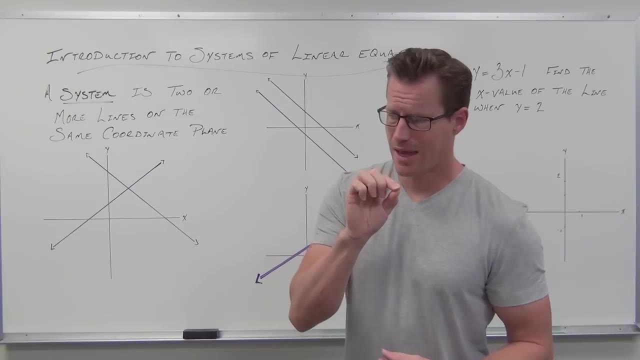 time. Remember the idea system means two lines on a graph. That's what we're looking for, Or two equations that make two lines in a graph. We're looking for where those lines cross. At most they can cross at one point. if they're not, 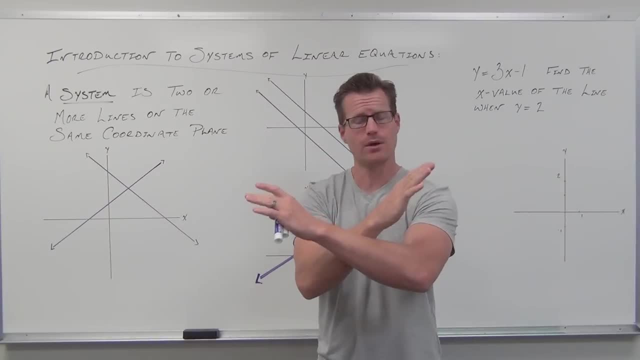 exactly the same line. These are lines. They don't come back and curve around, So that's what we're looking for almost all the time. is that one point that's common to both lines? That is going to be the solution to a system of linear equations? 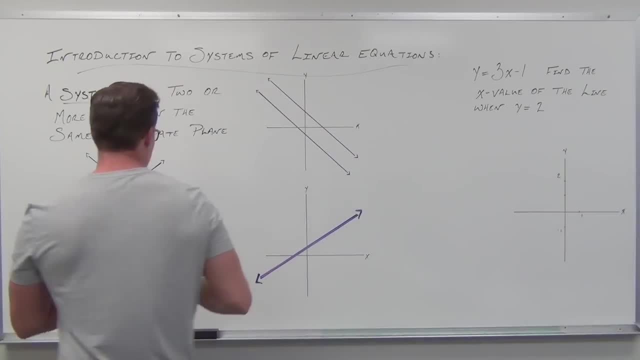 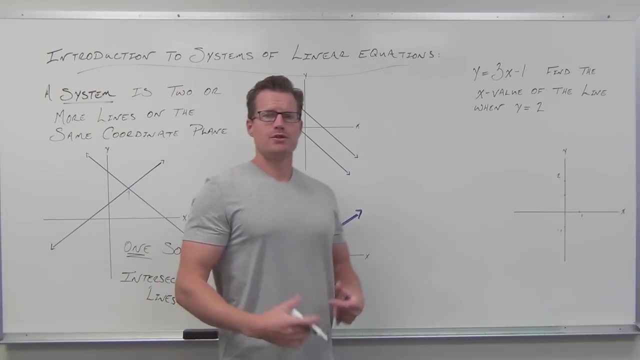 The one point, that's on both lines. So this would have what we call one solution. It's the point where they intersect right there. This has one solution and that's what our line is: Intersect. Could you have no solutions? Yes, we just talked about that. If your 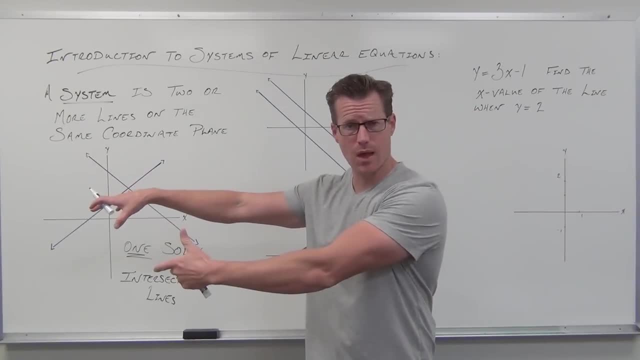 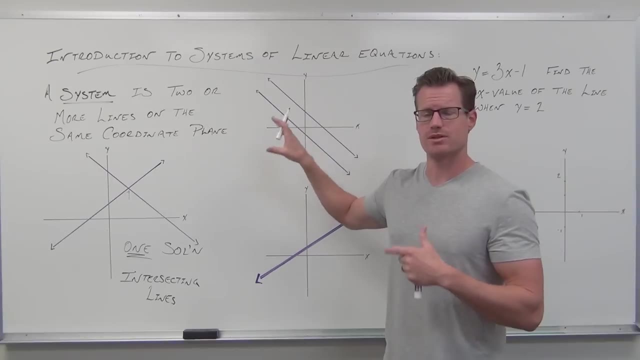 lines never intersect and we're looking for the point where our lines intersect. well, they're parallel. They never. they never do that. This would have no solution. So if you have the lines with the same slope, they're the same. 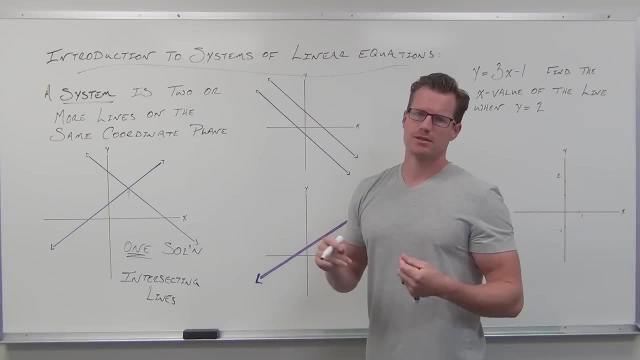 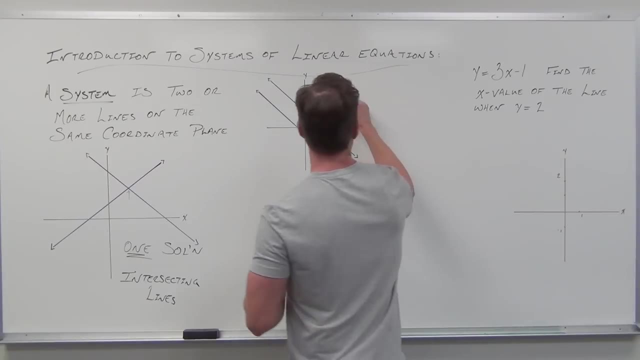 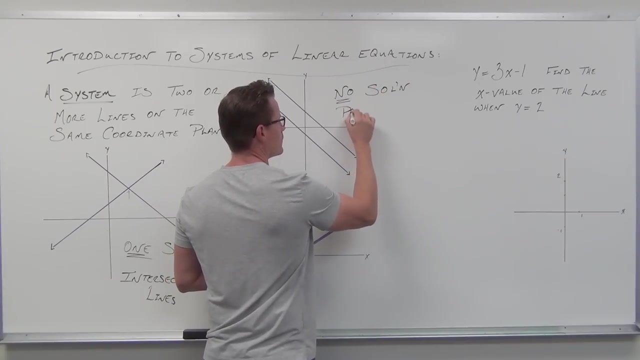 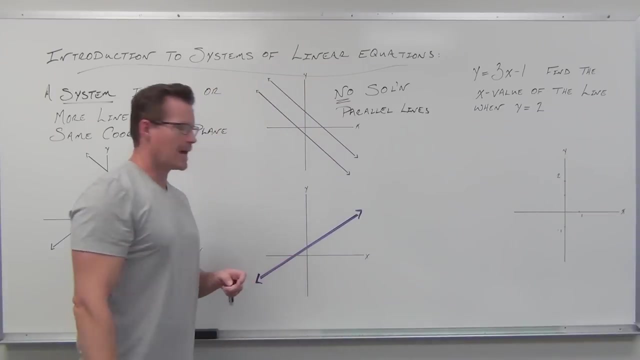 same rate of change, They're not going to intersect. Parallel lines don't have a solution for systems of linear equations, because we're looking for the point where these two lines intersect. Lastly, if you happen to have the same line and you might be wondering how in the 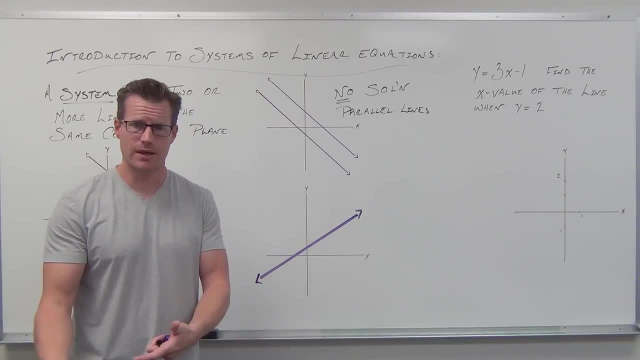 world. would you ever do that? I mean, wouldn't you obviously know whether something's the same line or not? Well, not necessarily. When we have everything solved for y, like slope-intercept, absolutely, You would notice that you'd have the same line twice. 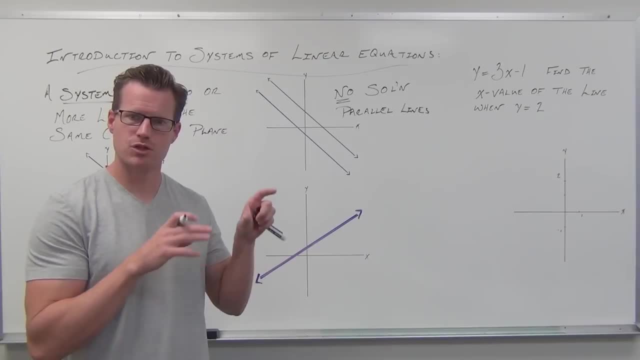 But in our intercept method you could conceivably have two different looks for a line. So maybe multiply everything by the number 2. You'd get a different look but it'd be the same line, And so conceivably we might accidentally graph the same line twice, one right on top of each other. 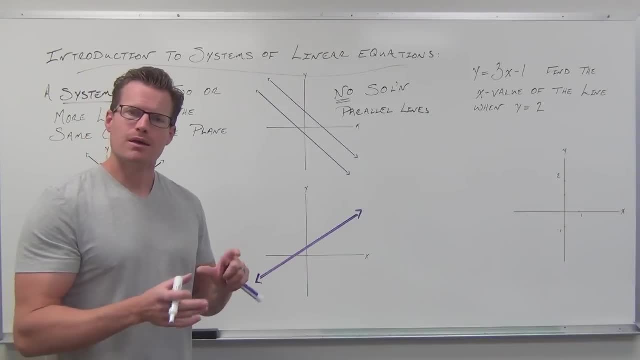 It's going to be very obvious: You're going to have the same line. In that case, when you've graphed the same line twice, of course they lay right on top of each other. So every single point would be common to both of them, not just one of them, not none of them. every point. 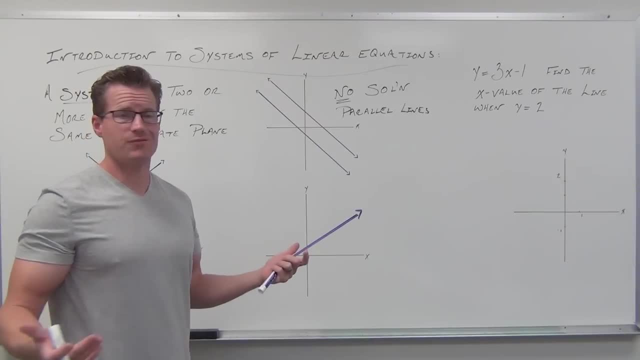 Well, how many points are on a line? Well, there's an infinite number of them, So that would have an infinite number of solutions. Every point would be common to both lines, because they'd be the same line. This would be infinite solutions. and that's when you'd have graphed exactly the same line. 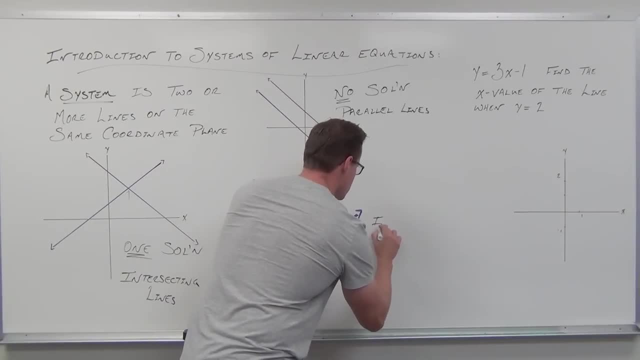 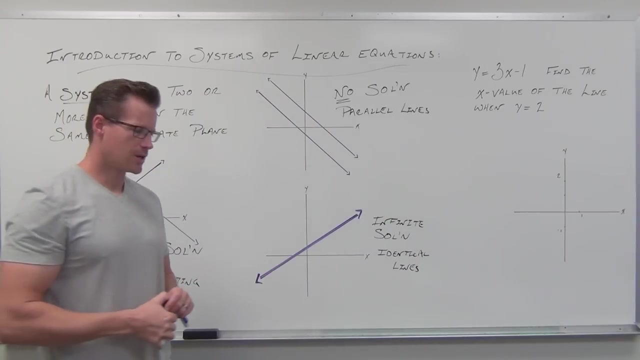 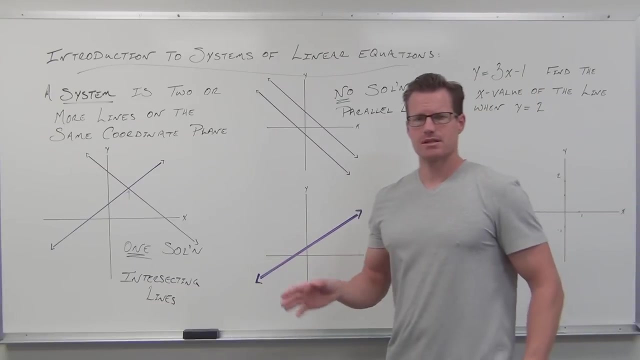 So that's really it. That's the introduction. Now I'm going to go through an exploration over here to show you exactly what we're going to be trying to do here. But that's what a system is. A system, if you just want a 30-second recap, what a system is is these two lines that are put on the same graph. 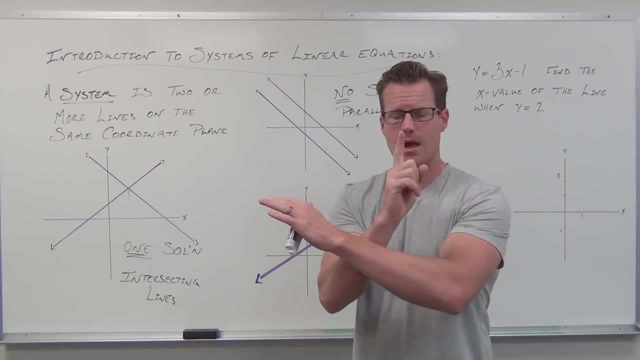 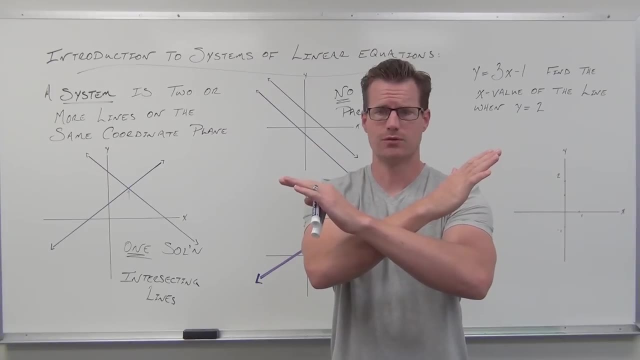 If they cross, they're only going to cross at one point. That one point is your solution to the system of linear equations. Where they cross is what we're looking for, because that's the only point that works. that's true in both equations. 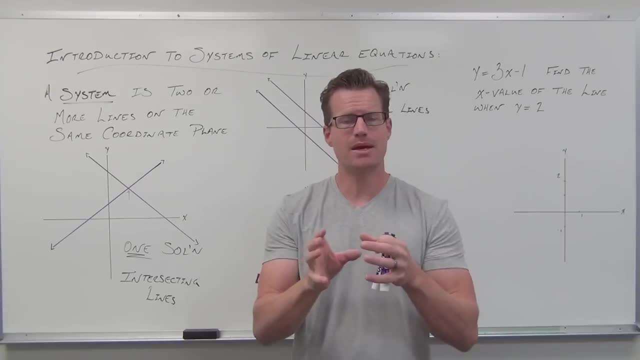 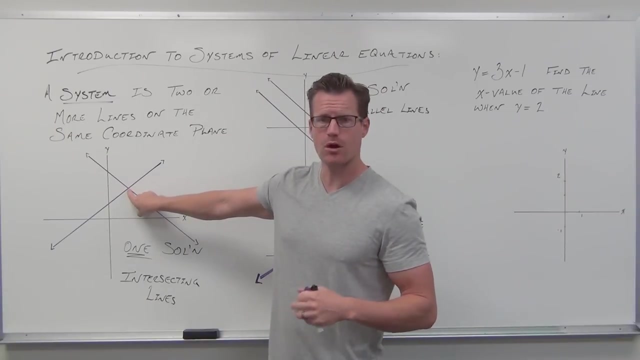 Remember what solutions are. There's these things that are true, that make a true math statement. So when we say I want the solution, I want the thing that works in both equations at the same time, well, the point that works in both equations at the same time is the one point that's on both of your lines. 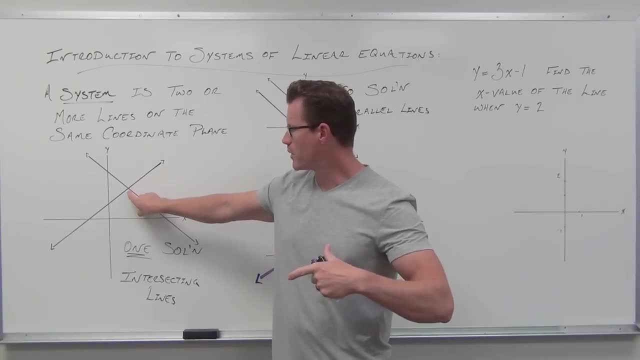 The lines come from your equations, So that point will satisfy both lines, It will satisfy both equations. and that's what we're looking for for systems: points that work in both: both lines, both linear equations, both equations. So that's what we're looking for. 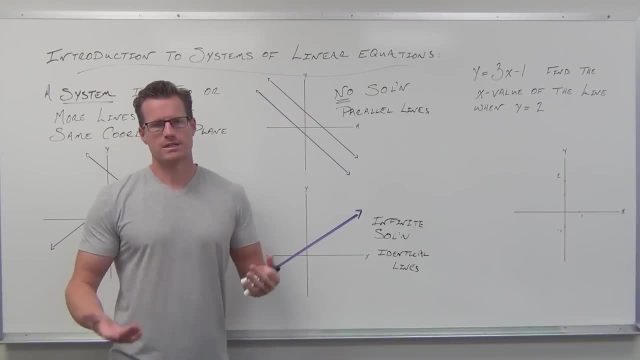 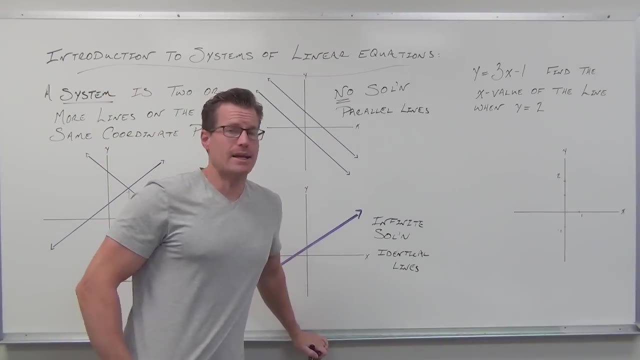 If your lines are parallel, you never have that. If your lines are the same, you always have that. Hence we have the no solutions, or infinite solutions. Now let's imagine something. Let's go on to our next example. Let's say I give you a line and at this point, man, you should be looking at it and going: hey, that slope is 3.. 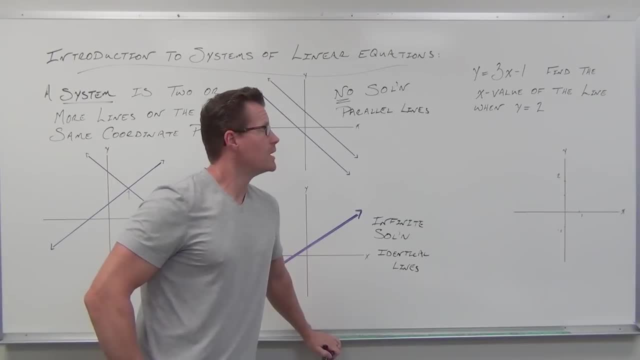 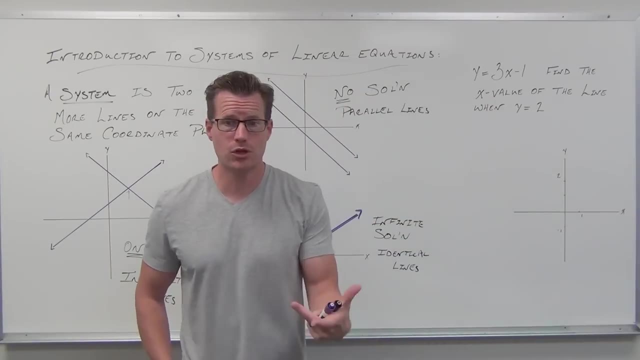 If that's not ringing a bell, you might go back and watch slope videos. Oh, and the y intercept is 0, negative 1.. It's right down here, So could you graph that line? I'm hoping that you could. 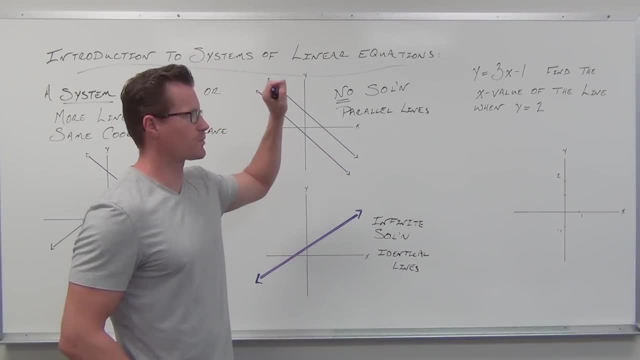 Be like: yeah, it's totally easy. I would go to the 0, negative 1.. I'd go up 3, write 1.. We're going to stop writing out a lot of that stuff, since you should be very practiced with it at this point. 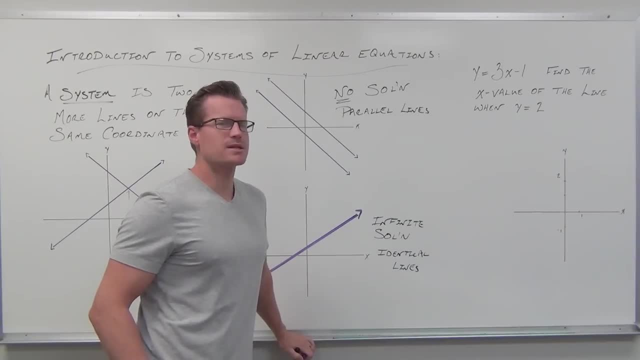 And then I want you to find the x. Oh, the x value. That's weird, That's different for us. The x value of the line when y equals 2.. Remember, I'm not just trying to have you plug in numbers and get the answer right now. 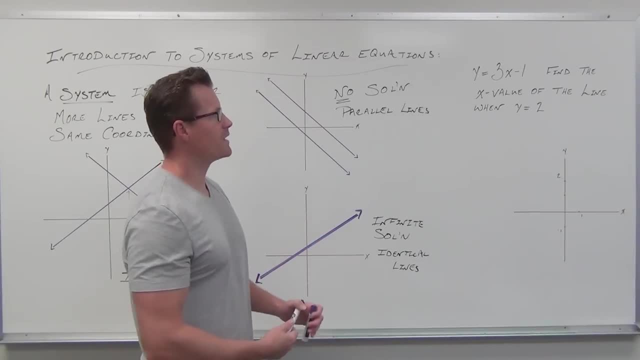 I'm trying to lead you to what we're going to be doing in the future. So if I have a line 3x minus 1, and I want to find the x value of the line when the y is 2,, well, I could do better. 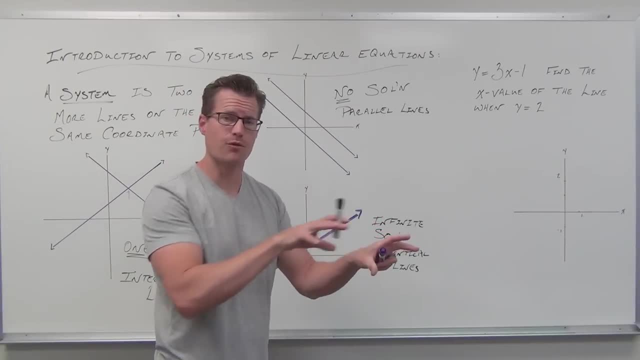 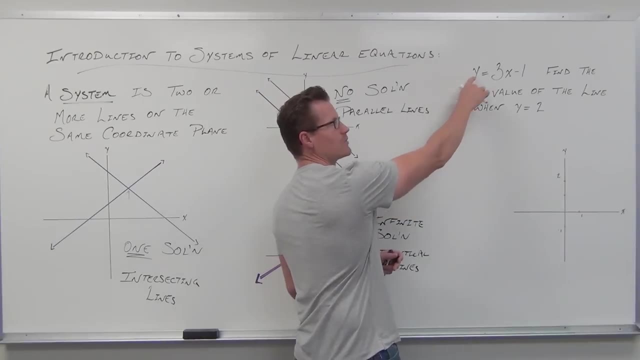 It's basically the same thing as it would when plugging in numbers to x and solving for y. only now I can plug in a number for y and solve for x, So let's try that. So, instead of y equals 3x minus 2, if I know that y equals 2, I could put the 2 right here. 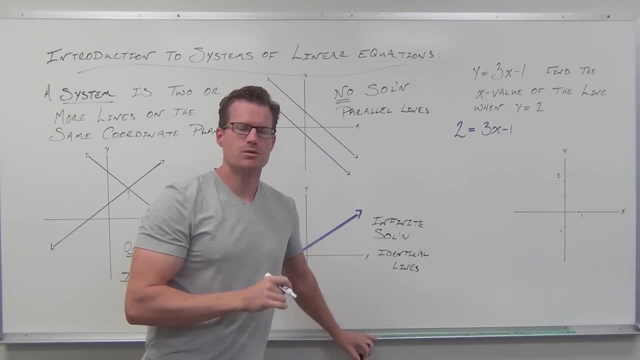 I'm going to ruin the suspense, I'm going to kill it. Spoiler alert: Did you notice what we did with the 2?? We plugged it in for y. We put it where y was. We substituted it in for y. 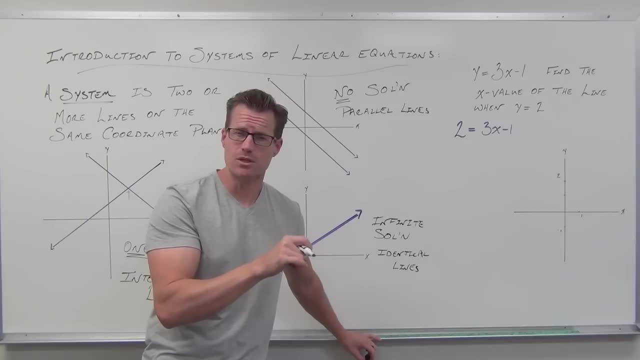 This right here leads to something called the substitution method. I get to it in a couple videos, But basically it says: if you want to solve a system of equations, this is a system of equations. y equals, y equals, That's two equations. 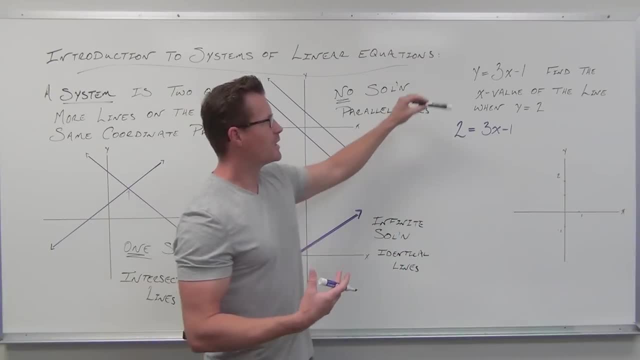 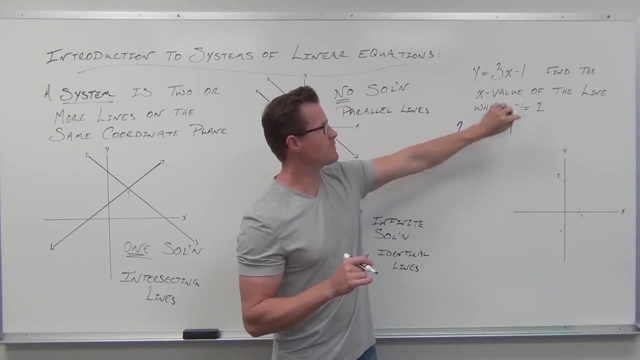 I'm going to prove it to you in a minute. when we grab it, It's going to be awesome, But you can always. You can always substitute the variable from one equation, what that equals, into the variable in the previous equation And by setting them equal, you can solve for the missing variable. 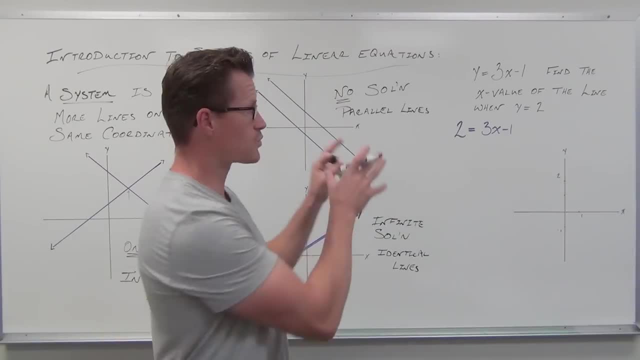 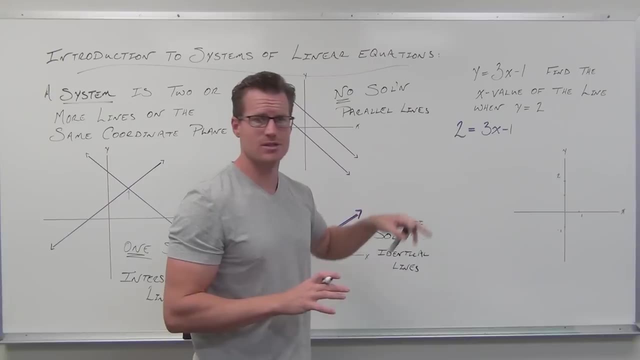 That's really cool. That's what the substitution method does. So this right here, this is going to lead us to the substitution method. I'm going to ask you, at the end of the example, which one's easier? You're probably going to say this one: 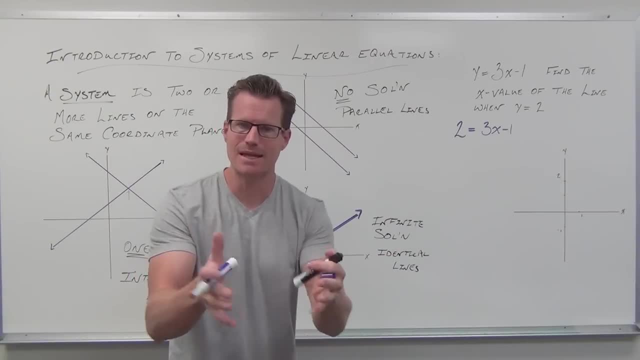 You're going to be like: yeah, substitution's easier. I don't have to graph Exactly. That's exactly what I want you to think, Because that's what we're going to be getting at, Because that's what we're going to be getting to is substitution method. 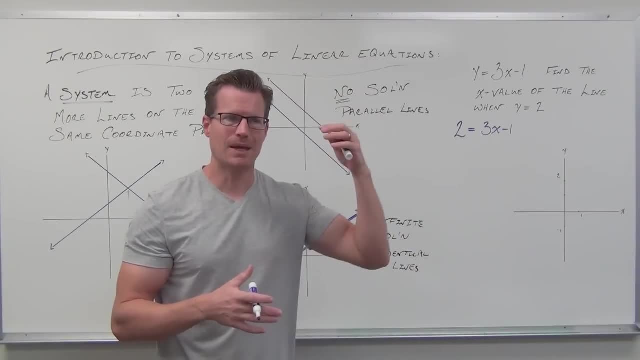 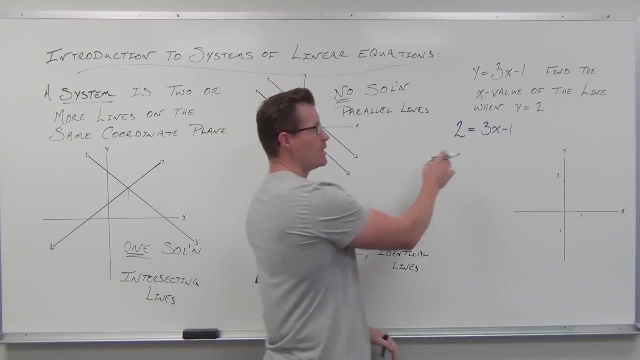 We're going to do a graphing method to really like pound in your head what we're doing, though, like what in the world these systems create for us. So we're getting there Anyhow. you can really solve that pretty easily if you add 1 to both sides and divide both. 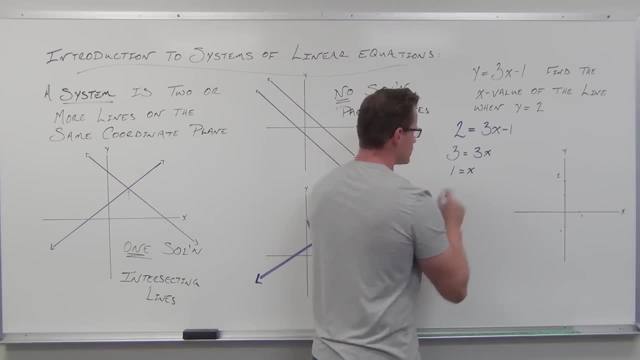 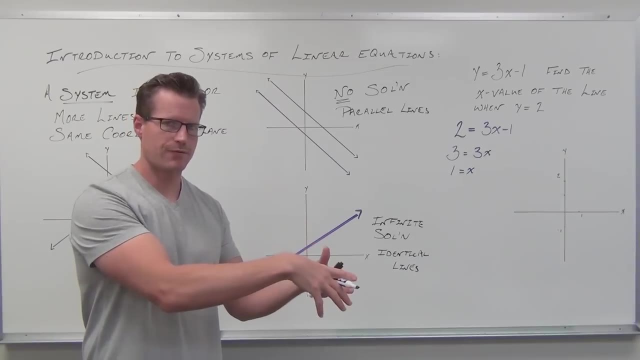 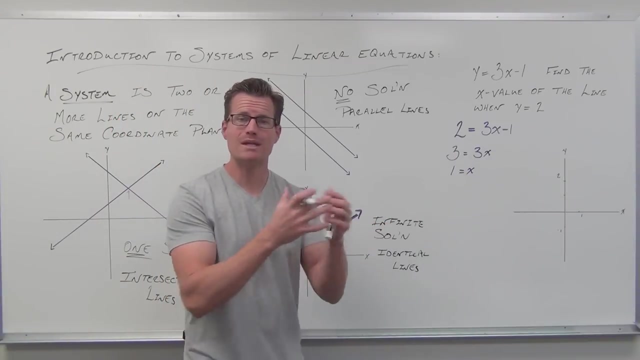 sides by 3.. x equals 1.. Now, because we're graphing, because I'm leaning towards graphing right now, And because these are lines, I want to write a point. So imagine that If I said, hey, y is 2,, I've already given you half the point. 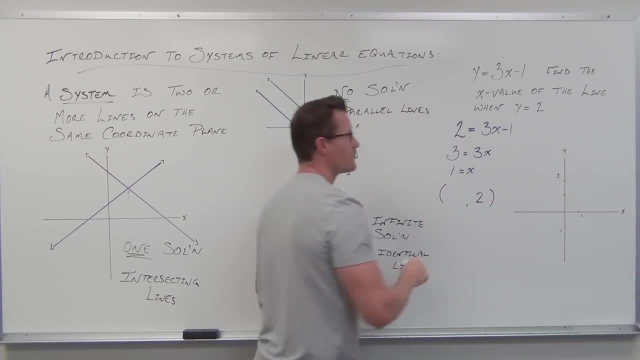 I've given you this y coordinate of y equals 2.. y equals 2.. Plug in 1 here for x. Obviously we're going to get y equals 2.. That's literally how we found x equals 1.. All we did was we solved for the first half of that point. 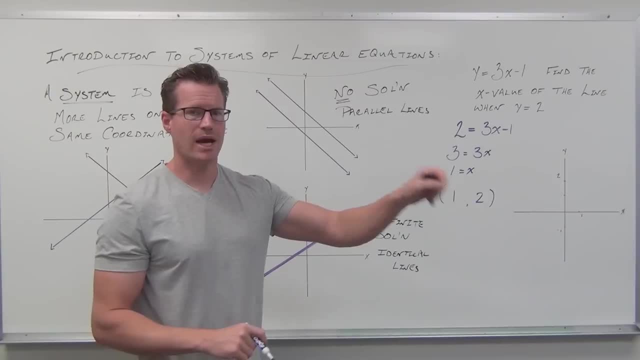 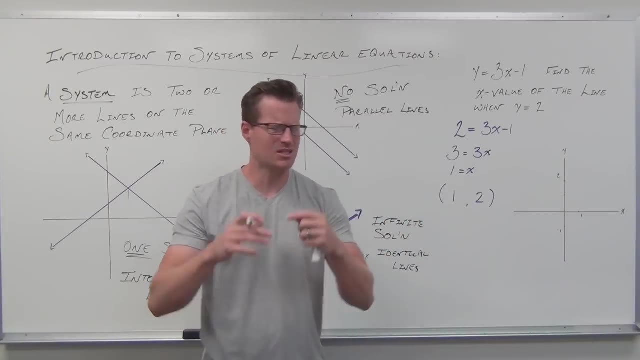 So now we know that when y is 2, x is 1.. And when x is 1, y is 2.. We have an ordered pair: x came first, y came second. Here's what this means. This is the whole point. 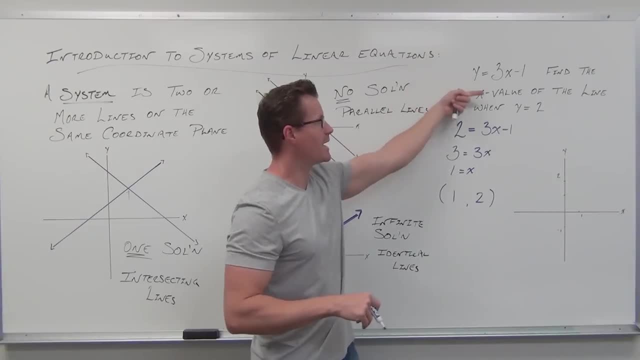 If this is a line- and it is, We just talked about it- And whoa Is y equals 2 a line? Oh my gosh. Well, does it have an x in it? I can't cross the x-axis. 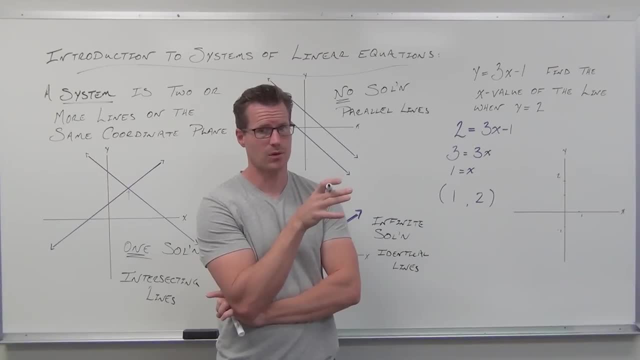 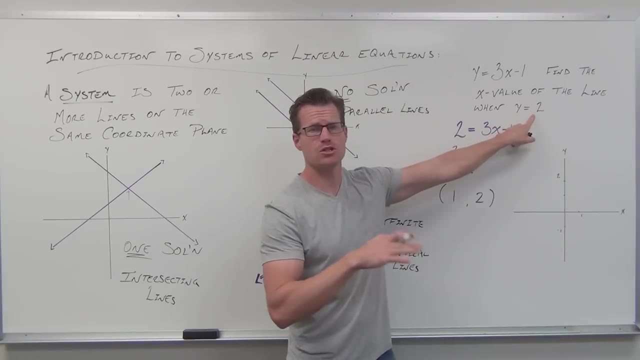 Slope would. if it doesn't have an x in it, slope is 0, if you remember that Slope is 0. That's a horizontal line. So wait, I know that I could do a substitution method. Plug in my 2 here. 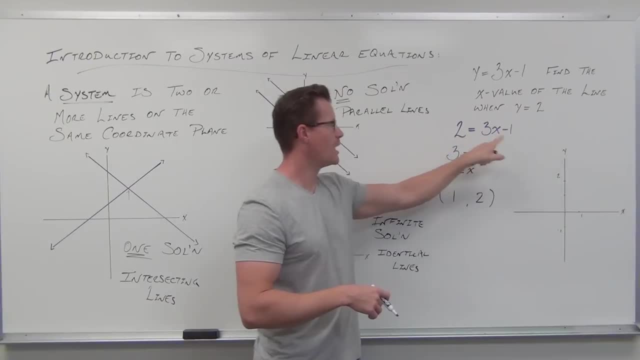 Solve for x. It's going to give us a point. I know y was 2.. I know that I could solve it and x is 1.. That creates an ordered pair: 1, 2.. But wait, What if we were to graph this: 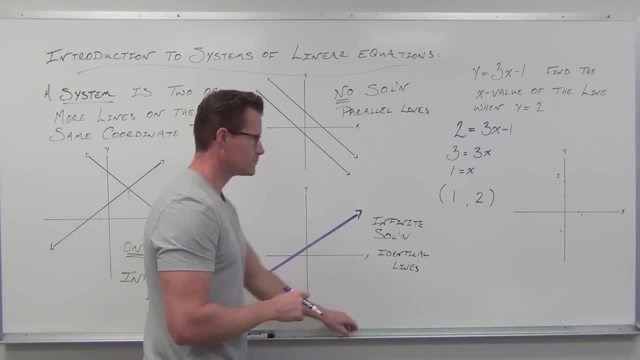 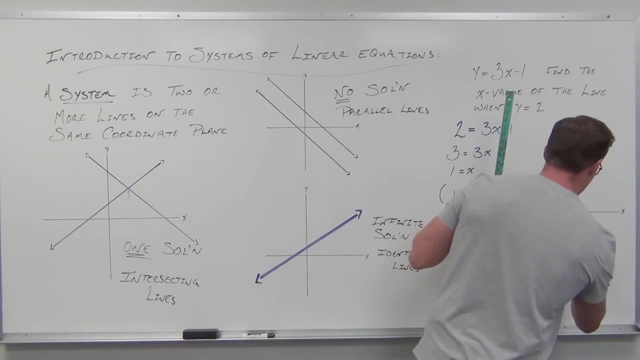 What if we were to graph the 3x minus 1?? So I know that my y-intercept is 0, negative 1.. That's what that tells me. I know our slope is positive 3.. So up 3, right 1.. 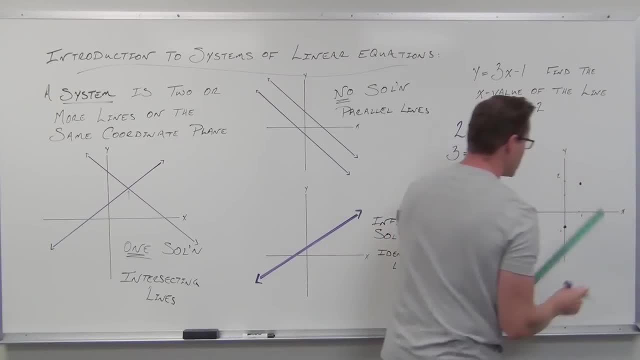 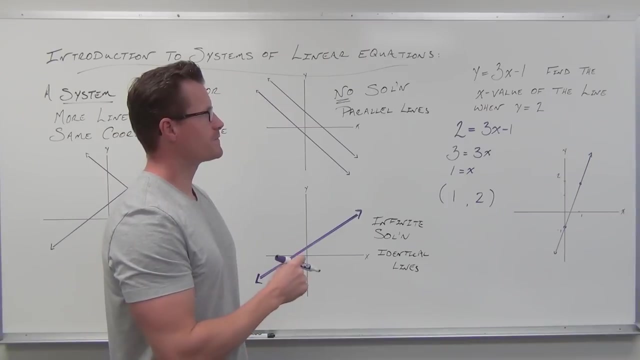 Up 3, right 1.. So that's our line, That's our first line. But then it says: find the x-value of the line when y equals 2.. But y equals 2 is also a line. y equals 2 is a horizontal line. 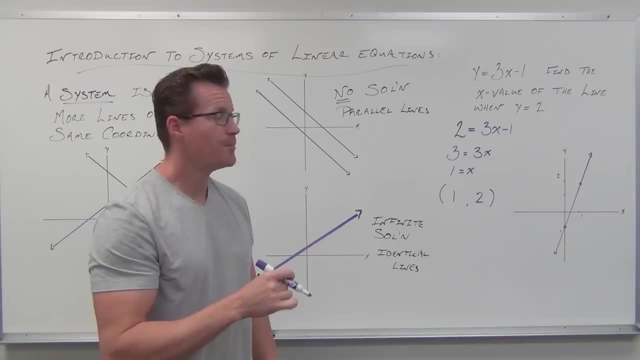 It has no x. That means the slope is 0.. It doesn't climb, It doesn't fall. It does have a y-intercept of 2.. It's given right there. It says: hey, no matter what, I don't care about you x. 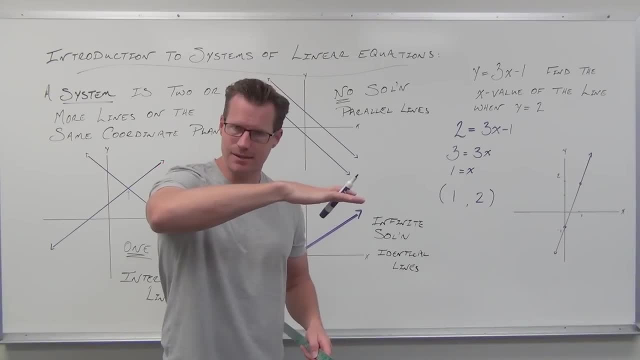 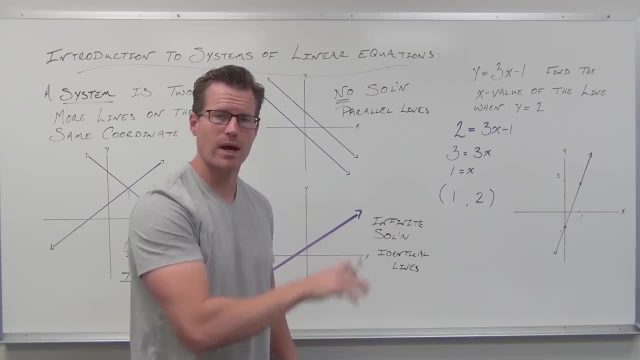 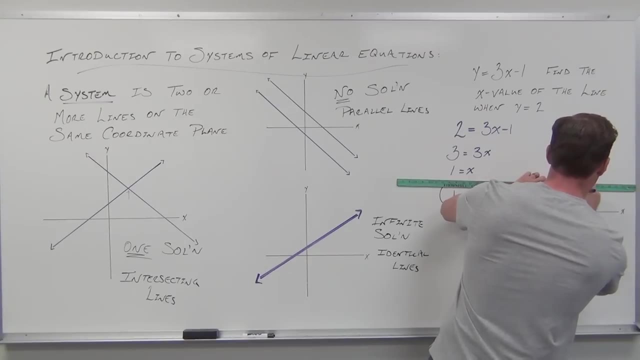 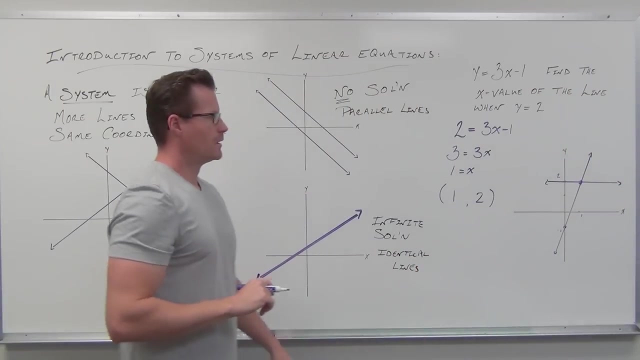 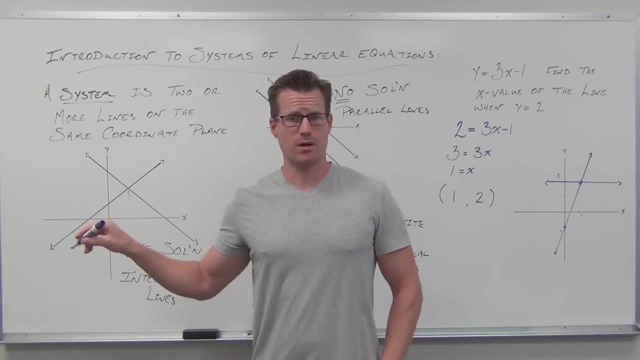 equals anything. i'm giving you out: two, that's exactly what y equals. two means it's a constant, that's horizontal. so the whole shebang, we unpack that and then we're pretty much done. you're looking for where your lines cross these linear equations. oh man, this is cool. 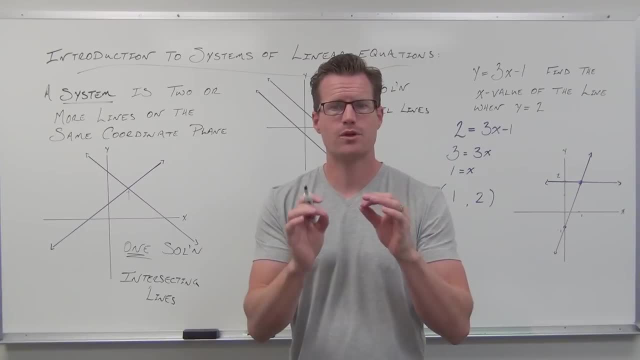 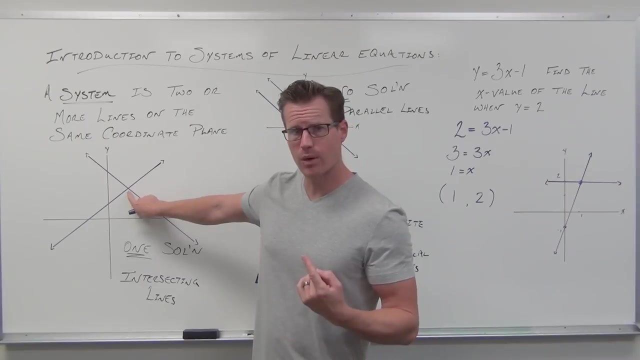 these linear equations make lines. we're looking for a solution, the one point or the points that work in both of them, the points that work in both, that are solutions to both linear equations are exactly the same as the point where they cross, because that's the one point that you. 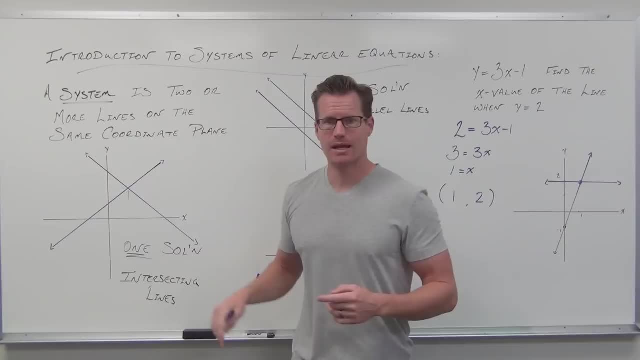 can plug into this line and this line and go, yeah, that's on both of them, that works in both of them. that's exactly what we've done. so if you graph your three x minus one and your y equals two, they're only going to cross at one point. then they're not the same line, they have to only. 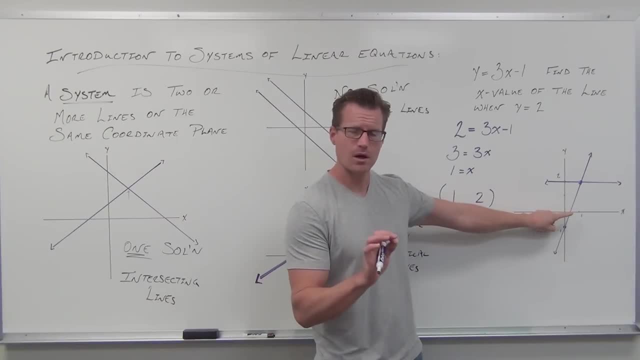 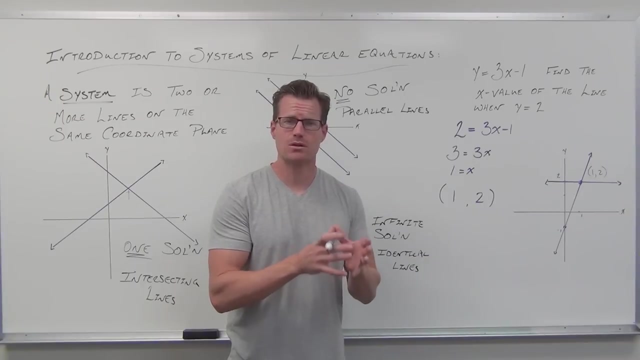 cross at one point, the point where they intersect. this is a big deal. the point where they intersect is the point one, comma two. it is no coincidence we get the same point. that's literally exactly what we're doing. so the point where your lines cross is the solution. 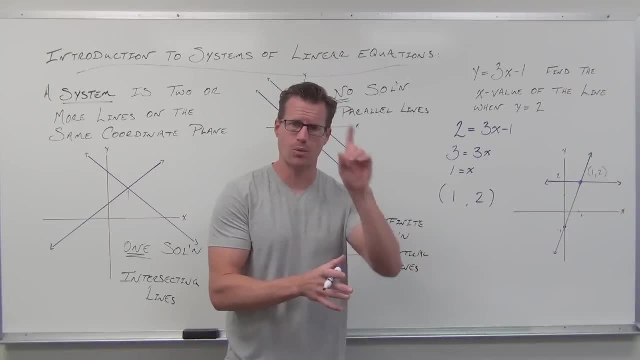 to the system of linear equations. that's what we're talking about, the one point generally, the one point that works, that is on both lines. if you have one point that's common to both lines, those lines intersect at that point they have to these points. that's not common to both. that's on. 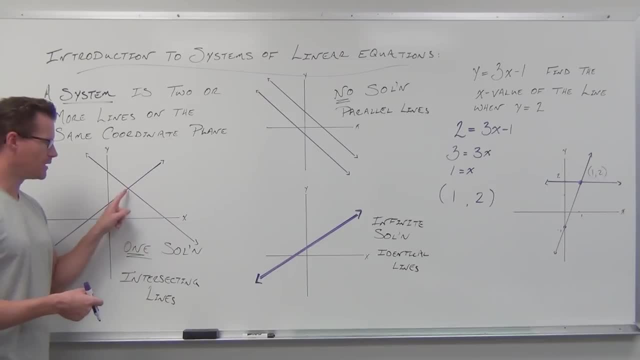 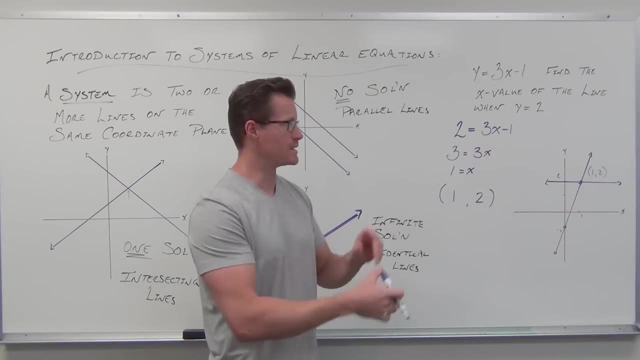 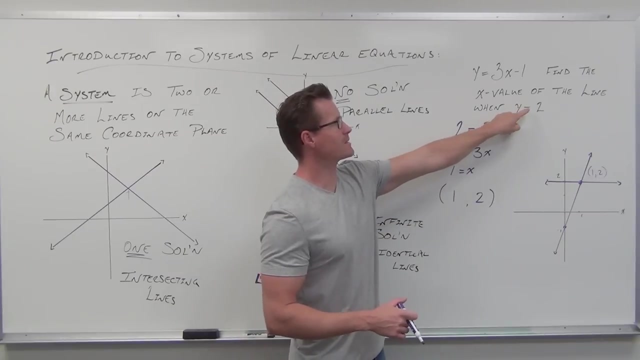 one line that's not common to both. that's on only one line that's common to both. that point is on both lines. that's exactly what we're finding. so what we've hopefully gleaned from this whole lesson is this: there's two way, least two ways, to do this. number one way you can always substitute one equation into another. 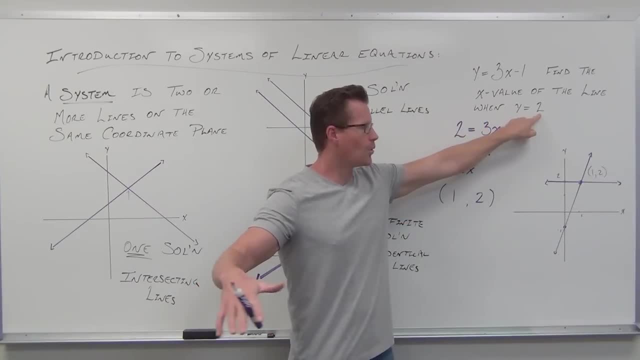 equation. so if y equals two, that means y equals two all the time. well, that has to make sense where our point intersects. if we're, if we're going to try to find the point that's on both lines- and i say this, one's always got to be two- then you're looking for a point on the other line. 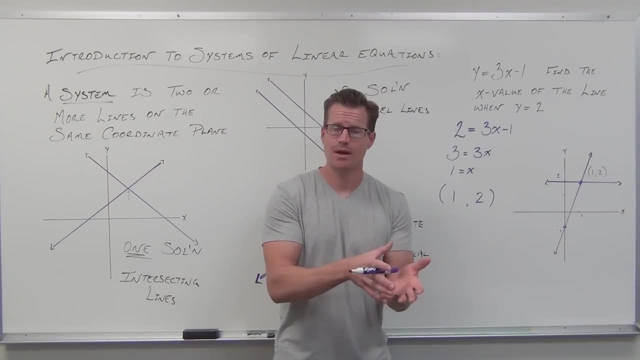 that has the same y value, that lets you substitute. that says, well, if the y values have to be the same, for that point, don't they have to be the same for that point, don't they have to be the same for that point. if i tell you a point is on both lines, well, their x values are going to be the same. 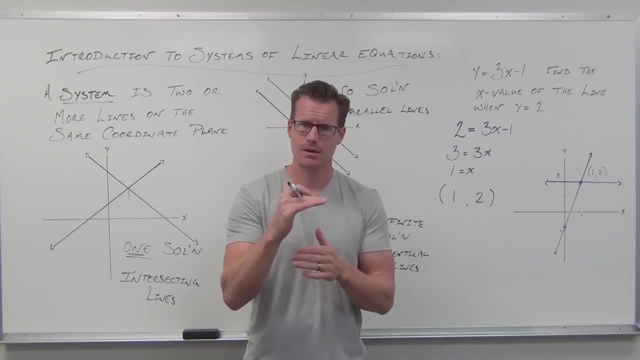 and their y values are going to be the same. so if i give you one line and say, hey, that's a, that's a y, your y is two, you go: oh, i'm looking for the. they're the same, let's let that y be the same. 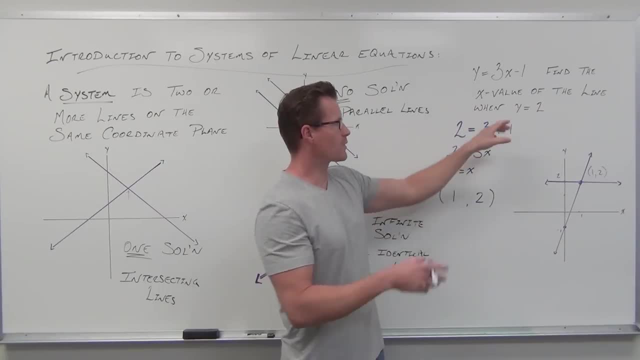 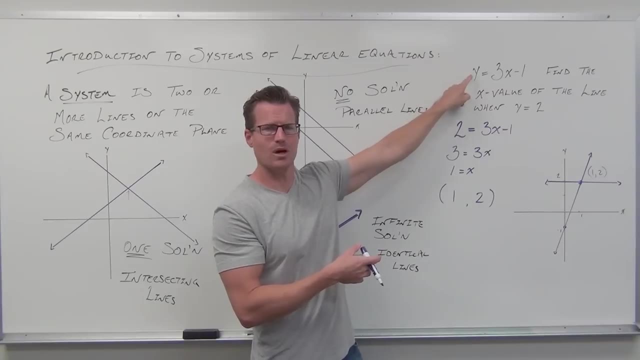 as that y. they're gonna have to be if they're the same point. if their y coordinates are the same, they're gonna have to be anyway. that lets you take that two and replace that y with two. that's cool, you're telling this thing. yeah, i'm looking for the point that has the same y coordinates.